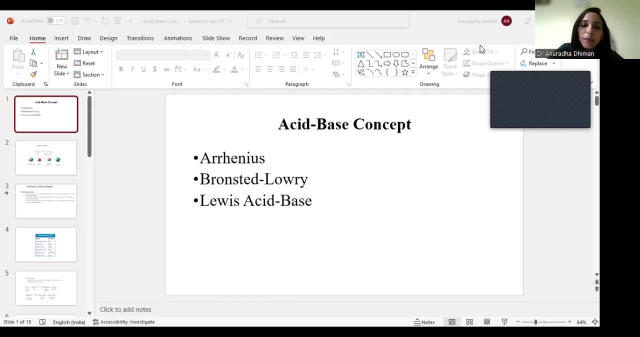 And, as we all know that, according to many schools of science, or, in my opinion, the, we may have some time that have a problem in English. and what do we have to do? we have also have to clear our understanding, which means we are not studying in English, but we 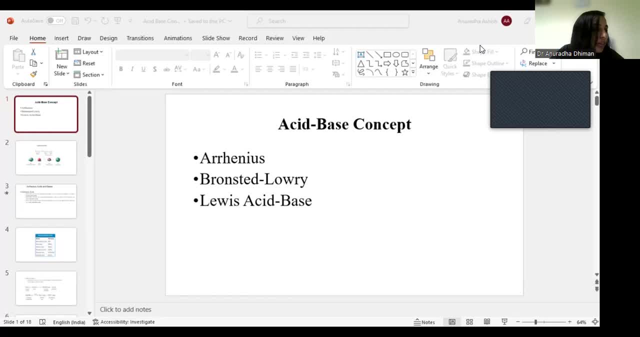 are studying chemistry only, So I thought, rather then learning English, I should only make in Hindi, so that more students can understand more easily. So what are agents and bases? If the pH in the paper is 0 to 40,, if its pH value is less than 7, then it is an acid. 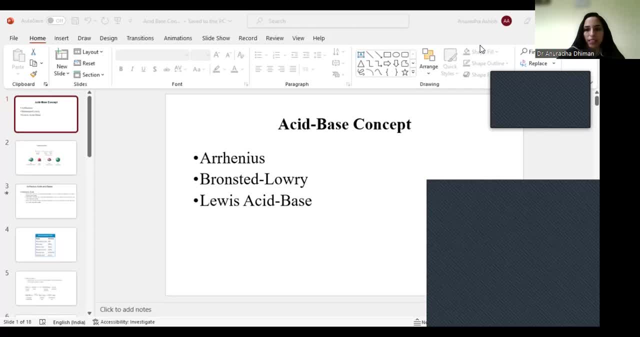 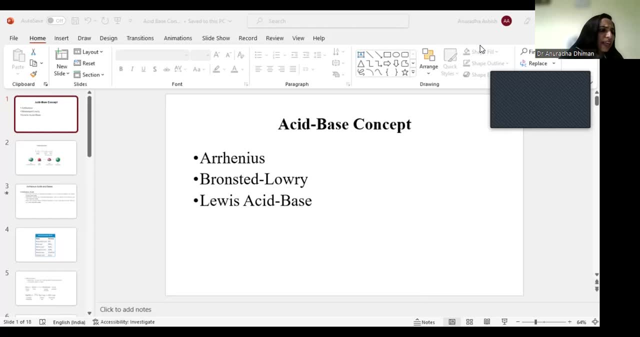 If it is more than 7, then it is a base, If it is 7,, then it is neutral. This is in the normal language. Now, according to the different theories, we can differentiate between acid and base. What is acid and what is base? 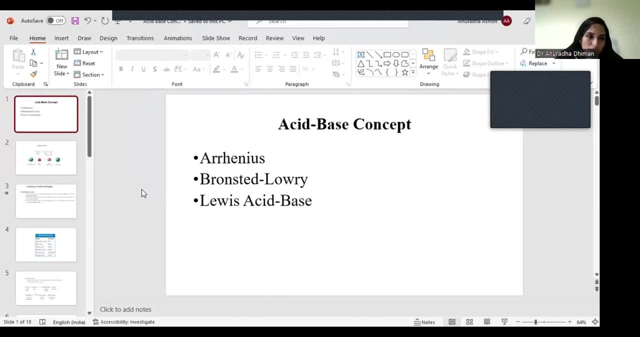 First of all, we will discuss the theory of Arrhenius. According to Arrhenius, what is acid? Acid is the one which we dissolve in water and the proton H-positive releases it. That is acid. Similarly, what is base? 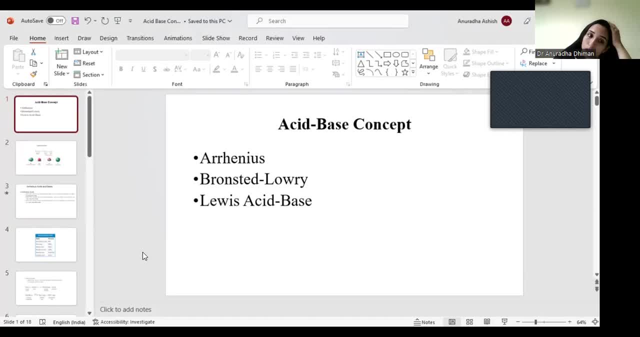 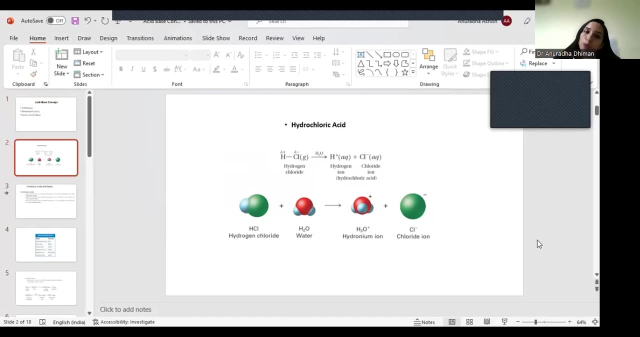 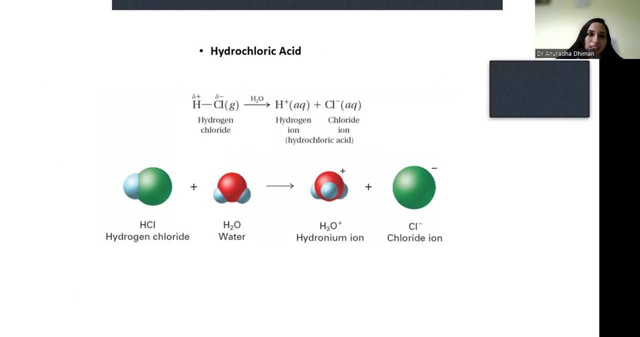 If we dissolve the base in water, then it is the hydroxyl ion which is OH- The acid will donate to H-positive And the base will release OH- It will release the OH- You can see, I have taken the example of hydrochloric acid. 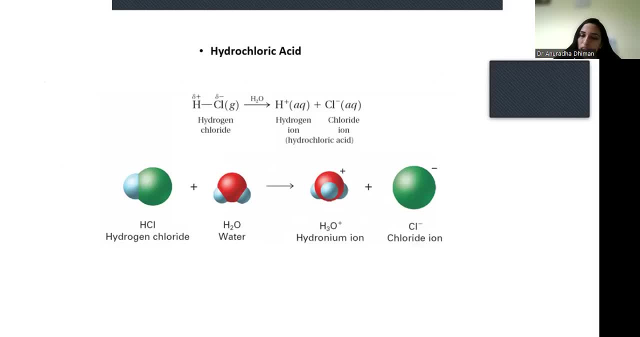 What is in this? It is H-positive. This is a partial charge. Maybe you have an idea. This is a partial charge As two atoms join together. One is H-positive and the other is C-negative. If I dissolve this in water, then it will release H-positive. 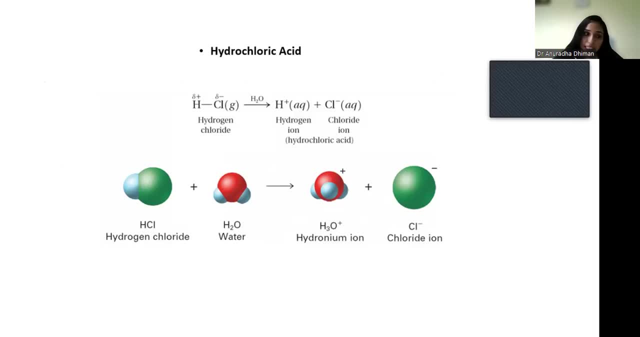 You can see. This is an acid. This is an Arrhenius acid. This is an acid. This is an acid. You can see below. I have taken another example. It is a hydronium ion. A hydronium ion is the same as H-positive plus H2O. 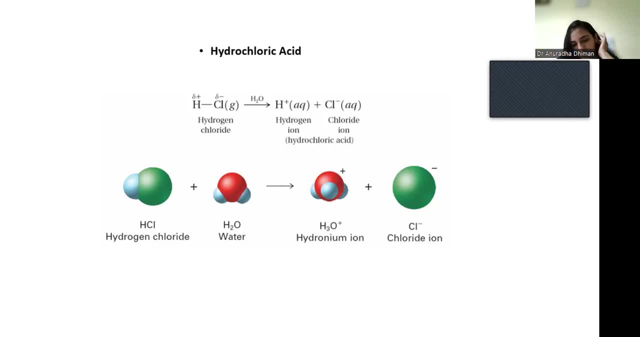 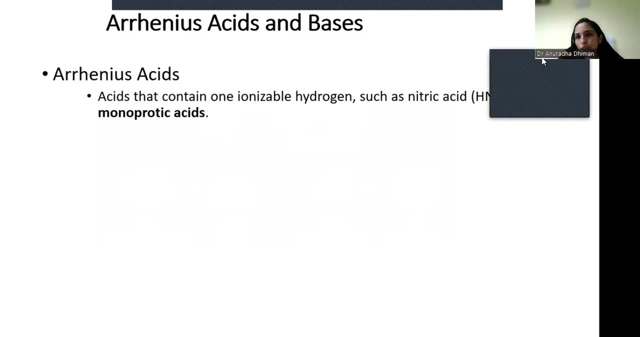 Okay, The difference is the same. The acid releases H-positive and the base releases OH- It is the same here We have discussed the example. We have discussed the same. We have discussed the same. what is acid With which? What is acid? 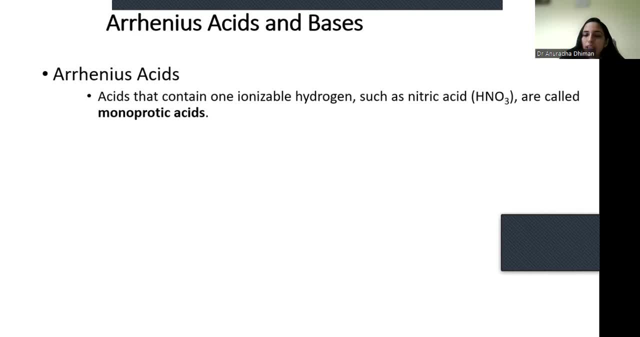 has one ionizable hydrogen. okay, How did it happen? Nitric acid- Now you can see that nitric acid has one H. H means H positive. So what will we call this? Monoproteic acid? What is monoproteic acid? It has one proton. When we put it in water, it will release its. 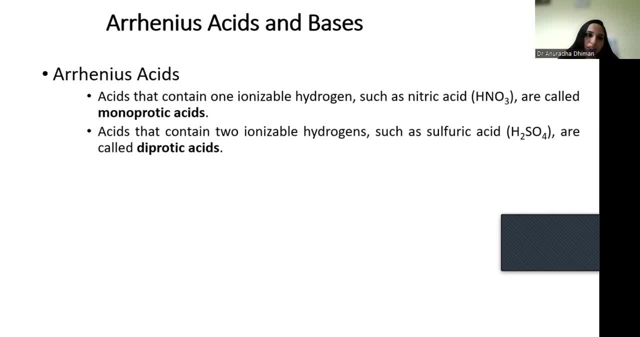 H positive, We will call it anionic acid. Okay, Now diproteic- what is it called? You must have seen sulfuric acid. You also know the formula of sulfuric acid. What is it? H2SO4. Okay, If we take the example of H2SO4, it has two ionizable hydrogen. So what will we call it? 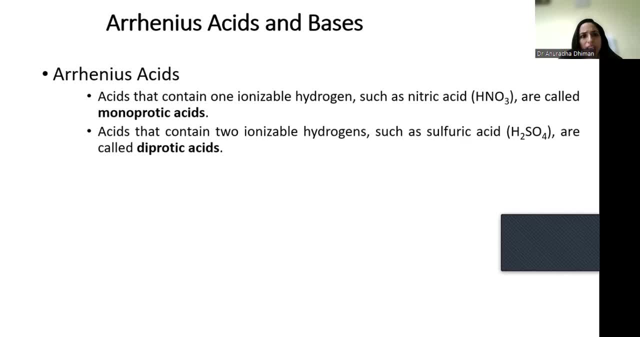 Diproteic acid. Okay, One is all-arginine acid, one is monoproteic, one is di and one is triproteic. What is the example of triproteic Phosphoric acid? What is in it? Three ionizable hydrogen. 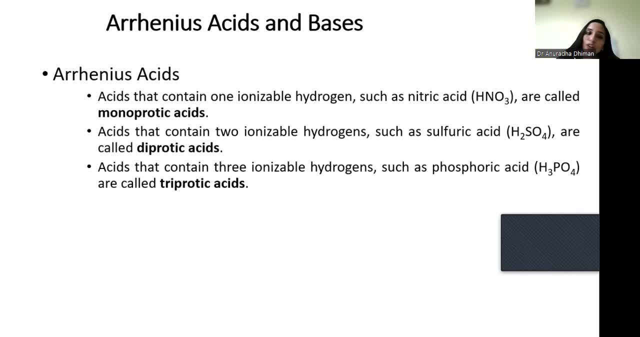 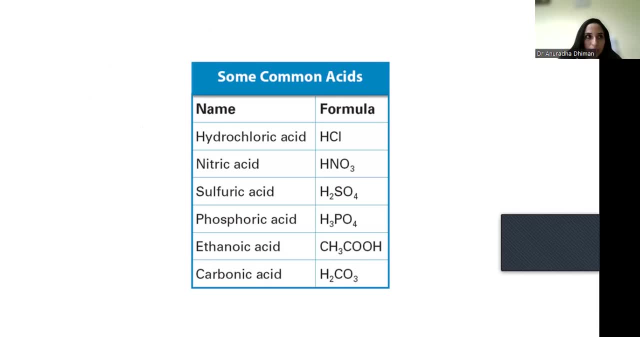 are there. Example of phosphoric acid is H3PO4.. What is it called Triproteic acid? Okay, These are all-arginine acids. This is a common example: Hydrochloric acid, HCl, then nitric acid, HNO3, then sulfuric acid, H2SO4.. This 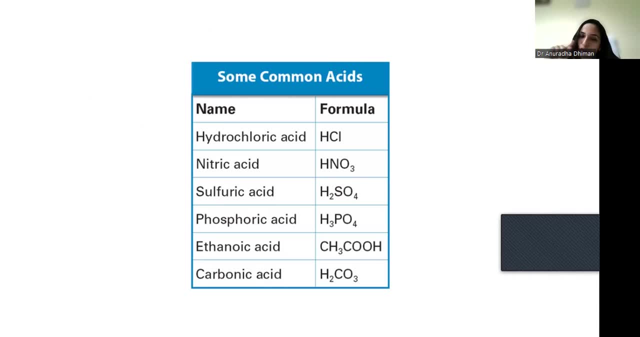 is your home practice. You make another column in front of it, Write on it which is diproteic, which is monoproteic, which is triproteic. If still there is any doubt, you can comment in the comment box. Fine, Or you can follow me on the Facebook. 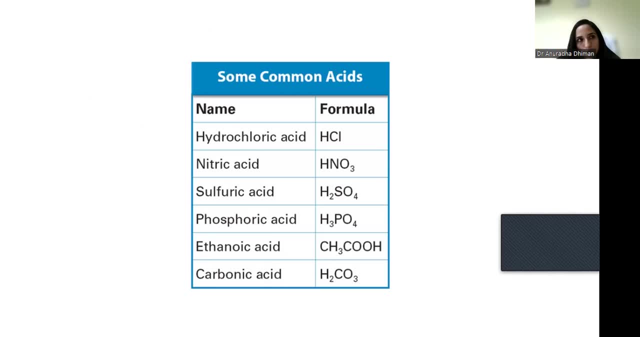 As well as on the Instagram. On the Facebook I have one closed group, Computer-aided drug design. You can join that. Generally, we discuss number of things there. Okay, Carbonic acid is there, Ethanoic acid is there. These are all acids. You can divide this in the classification. 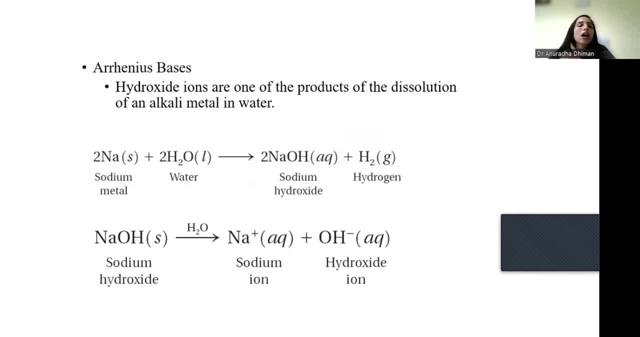 of Arrhenius acid, according to you. Okay, Now base is here, As I discussed earlier. what is base? It has hydroxide ion. Now when we dissolve it in water, it becomes OH- negative. When we dissolve it, it releases. You can see. this is I take that pen. It is in spotlight. 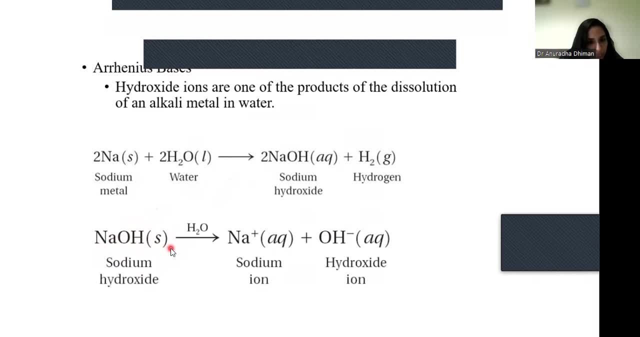 Okay, Look at this Here. it is NaOH. We put it in water, So what has it made? Na-positive plus OH- negative. Okay. Next one more example is sodium metal. What is there in it? When it is put in H2O, then it has made sodium hydroxide. This is the base, So this is the 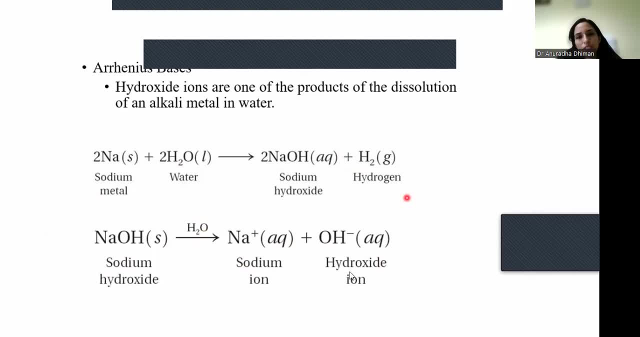 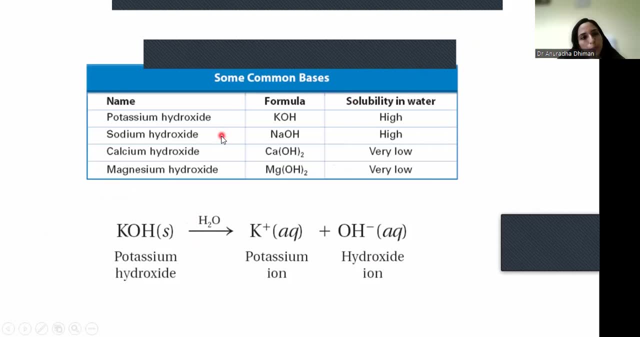 base. When it is dissolved in water, it will release OH- negative. Okay, Now what is this? This is a common base example. Now its solubility is also given with it. One is potassium hydroxide, sodium hydroxide, calcium hydroxide, magnesium hydroxide- All hydroxide you can. 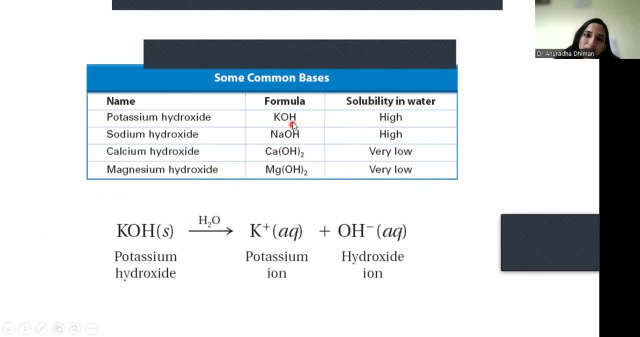 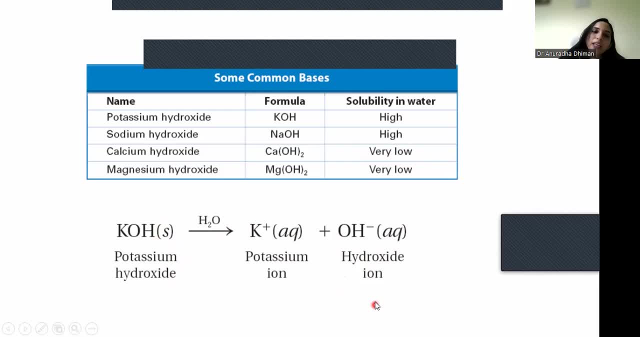 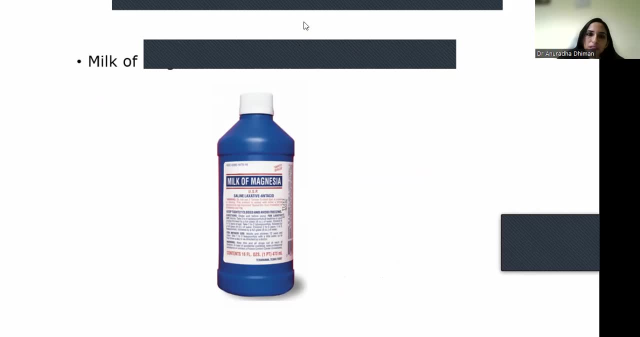 same. We put water in NaOH, So it released OH- hydrogen hydroxide. Okay, What has this done? Arrhenius has been based. Now this is milk of magnesium. This is the example provided, One simple Here again. Uh, milk of magnesium is also called the base, and in 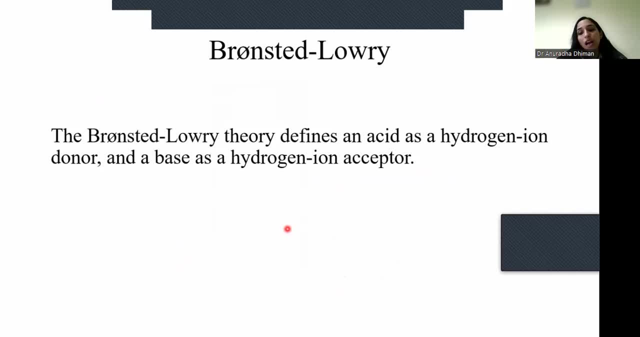 general, it is an antacid. Now second one, I will give it again. This is a very, very. It is used as an anti-acid. Okay, Our Hennius theory is clear. Is there any doubt in that? I think there should not be any doubt. 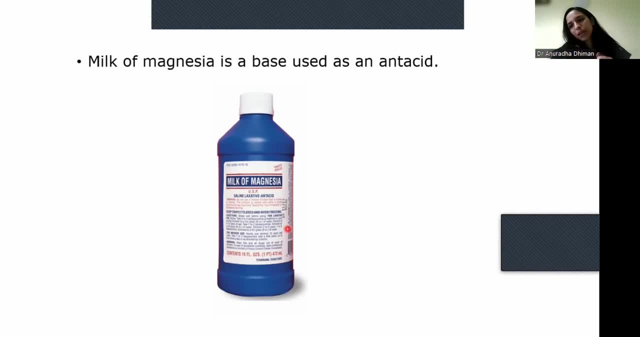 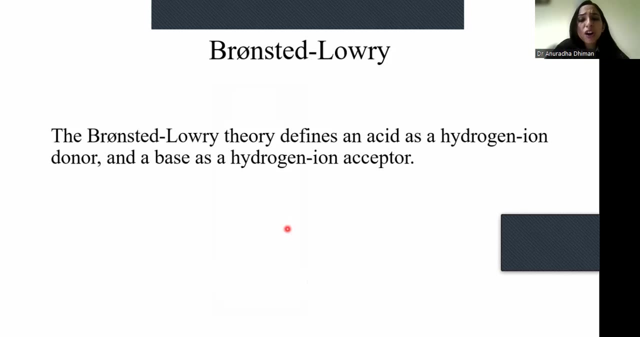 There is no doubt. If there is still any doubt, you can write in the comment box. We will discuss it again. Next is Rostel-Lowry theory. According to it, what is acid? First, we did what is acid? 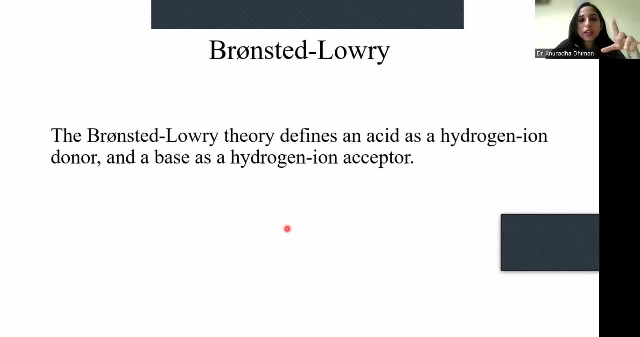 It releases H positive When we dissolved in water. what was the problem? in that We cannot differentiate every acid base like this Which is not soluble in water. So this was a big problem. So after that, Rostel-Lowry gave another concept. 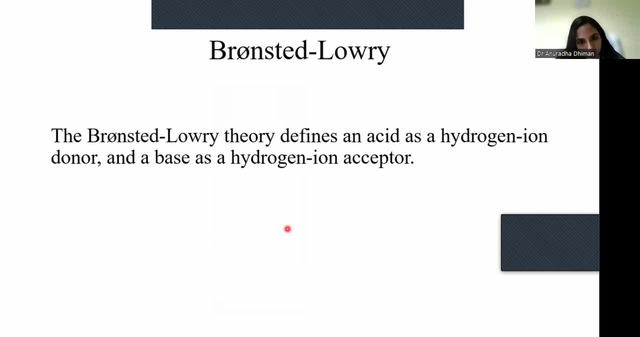 What is acid? The hydrogen ion donor, we will call it acid. And the acceptor, what will that be? It will be base Donor. you have heard I donation blood donation. Donor means you know it is clear. 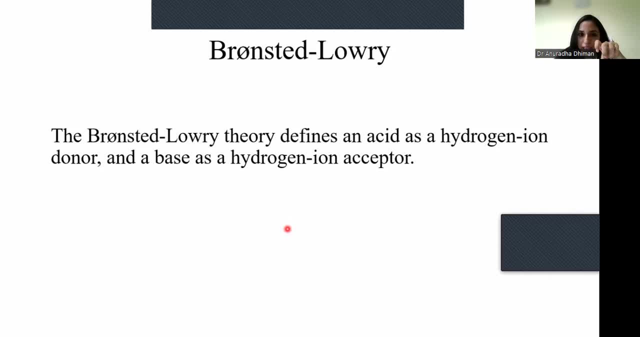 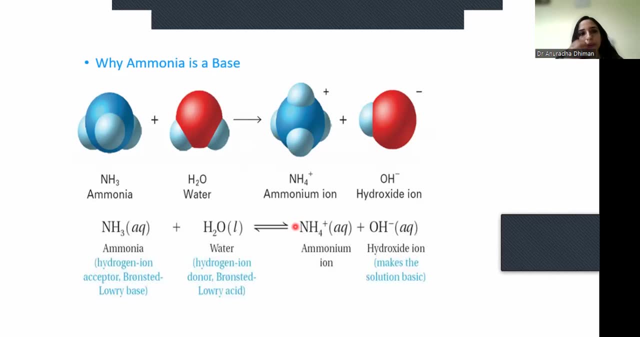 Donor means give. Donor means give to someone The H-positive ion. if it is given to the acid, then it is acid. If it is taken, then it is called acceptor Or it is called base. Okay, 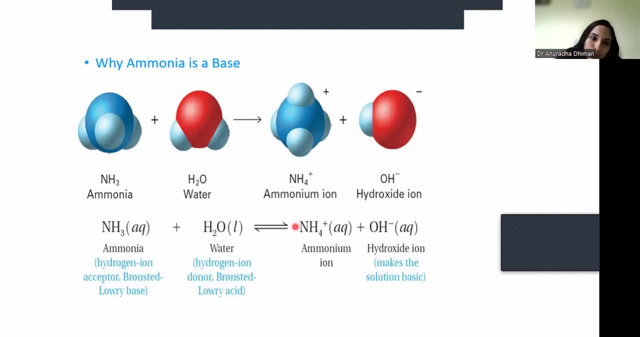 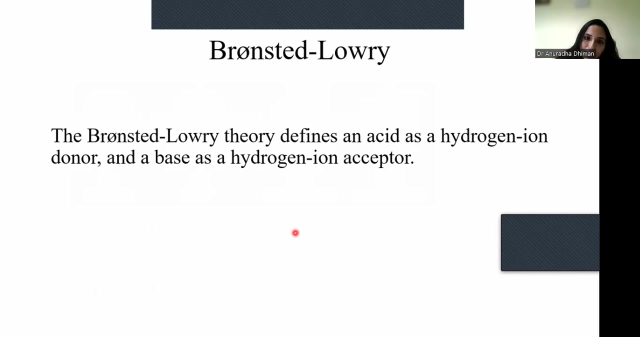 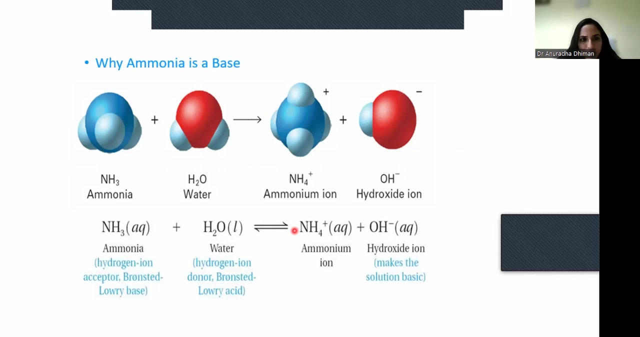 This is an example of ammonia. Now, why is ammonia base? Because what is this? What did we do? Donate, Okay, So in this concept, the ammonia should have been a hydrogen ion acceptor, right? You can ask this question again and again. 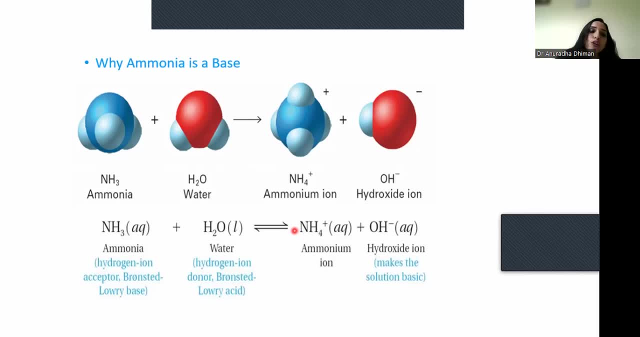 Why ammonia is base. Okay, What will you write in that? Because the bra. according to this, like we had written the first concept, Arrhenius. according to that, we were saying that the base will release the OH. 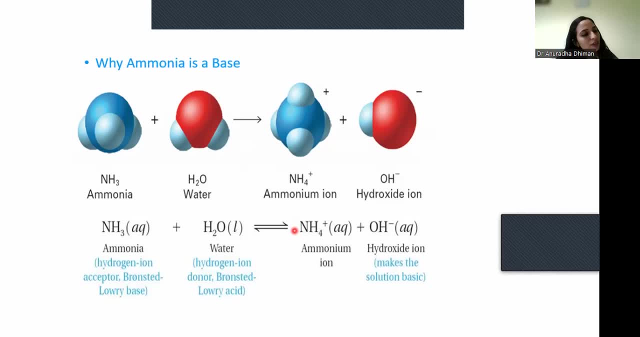 Okay, But the ammonia it does not have. OH, You see, the formula of ammonia is NHT. Okay, It does not have base. So the second concept, Laury Bronsted. it has satisfied it Because 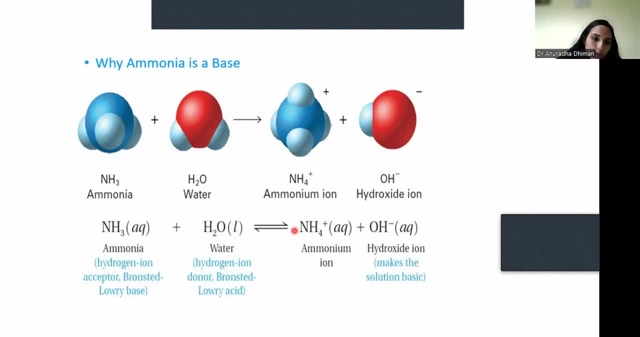 according to this, the hydrogen bond acceptor we will call it base, Okay, And the donor we will call it acid. If you ask this question, it is a simple question, Like we say that the base is that. 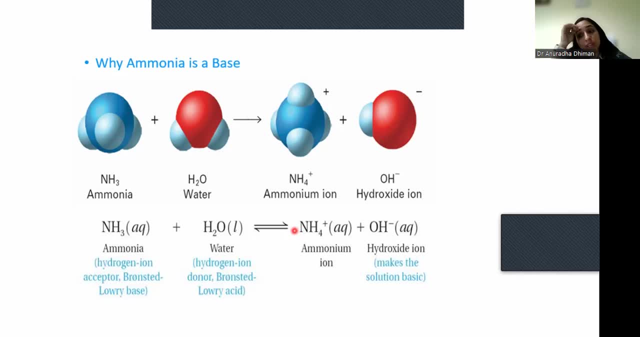 which will release OH. But you see, ammonia does not have OH. So why will we call this base? We will call this base according to Laury-Bronston concept. Bronsted-Laury has written in the concept that the base 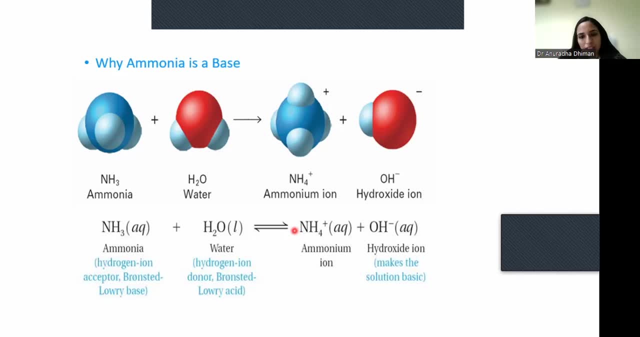 it accepts hydrogen ion. Okay, That is its Nana. it will baby this crust A 900.. Tiny Civic, So the next concept of acid. so, as you, As I said, we explain reason for the existence of acid. 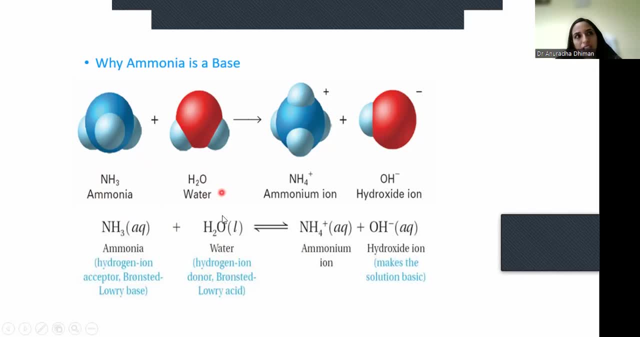 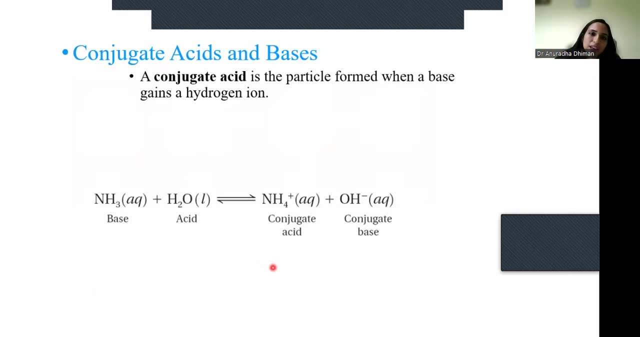 Thank you very much, Jessica, for responding. We will read the second part of it later on, but after all we need only 6 days to explain the way for hot and shaking of OH. He is telling us she has not added a lot of water to the bacon and the egg, with clue one. 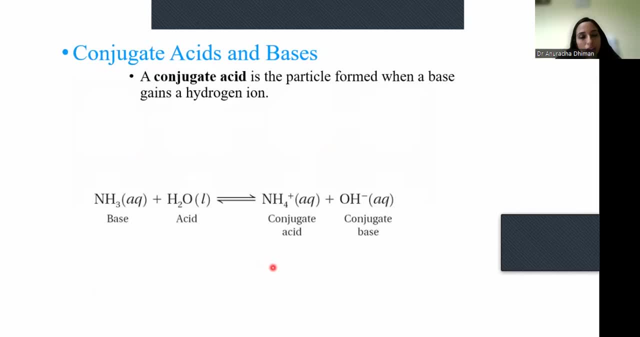 that's why we need water and a lot of ice for this time. What is a conjugate acid? When there is a base, it takes hydrogen ion. it is called a conjugate acid Like Na3 positive. Now, what is Na3 positive? 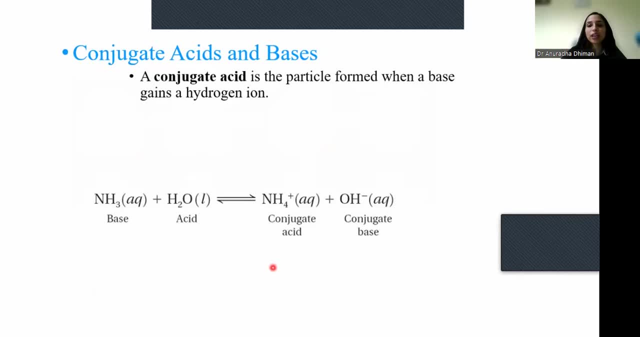 If it takes an H positive. it is called a conjugate base, It is called a conjugate acid. Remember: the base will become a conjugate acid And the acid will become a conjugate base. Both are opposites. What is a conjugate base? 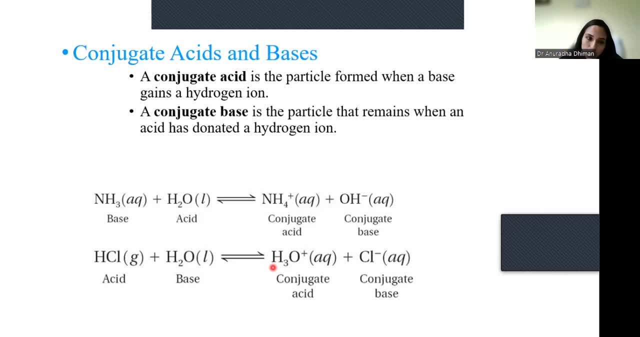 An acid has donated a hydrogen ion. it is called a conjugate base. Now see, you have given this example. If HCl is donated to this H, then it becomes a conjugate base. What is the opposite of it? This is a base. it has accepted an H, so it becomes a conjugate acid. 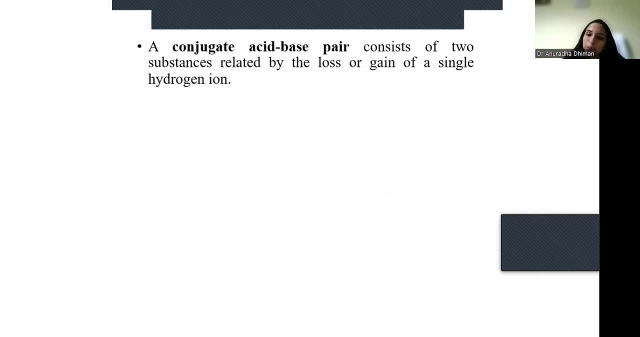 Okay, Simple, Now conjugate. What is a conjugate acid-base pair? Do you know what a pair means? Like we say, we have two pairs of shoes, One pair of socks. Pair means they come in pairs. Now, if an acid and base are a pair, what do we call it? 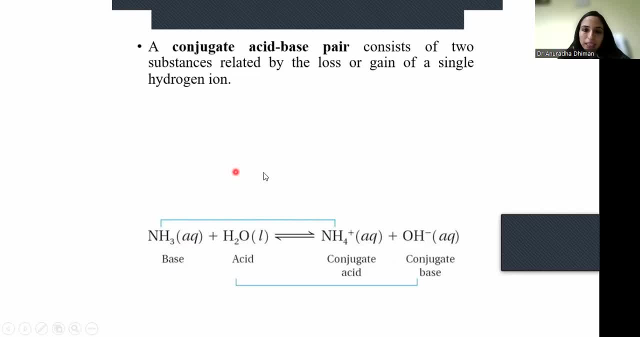 Look at it Now. what is this? It is a pair Base and the conjugate acid Consists of two substances related by the loss or a gain of a single hydrogen ion. Now see what is NH3-positive. It will take H-positive, okay. 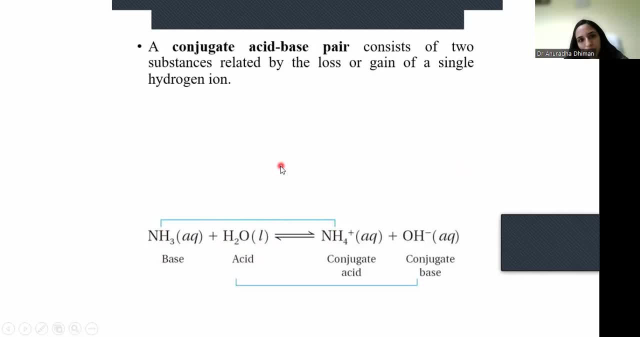 And what will it give? Now, what happened? The activity is balanced. The single hydrogen ion: one donated it and the other accepted it, So we called it a conjugate acid-base pair. And this substance, the substance that can act as a base as well as acid, that is known as anthroteric. 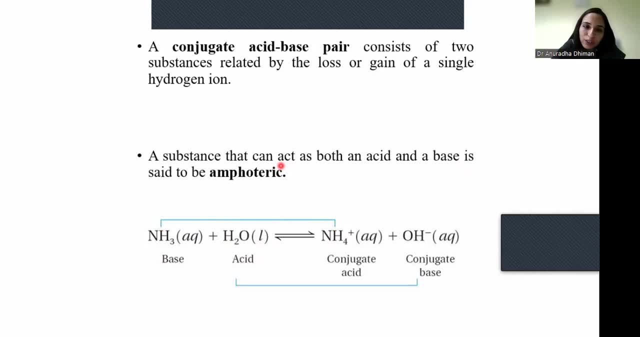 Remember, write it in a notebook. What video will you open again and again? Because these are important things. If you want to learn chemistry in depth, then amphoteric is important. What does amphoteric mean? Substance that can act as acid as well as base. 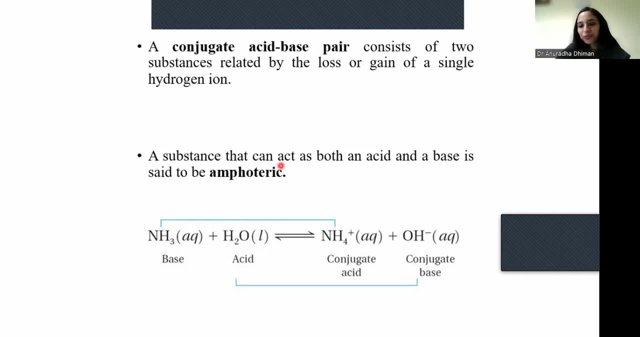 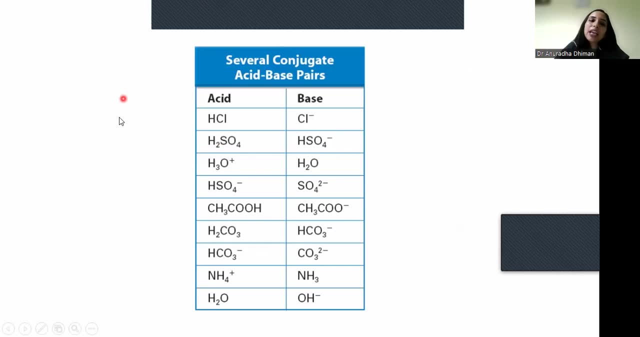 That is known as amphoteric Example. you will tell In the comment box what will be this example: Amphoteric- Okay, These are several conjugate acid-base pairs: HCl, ClN2.. Sulfuric acid. 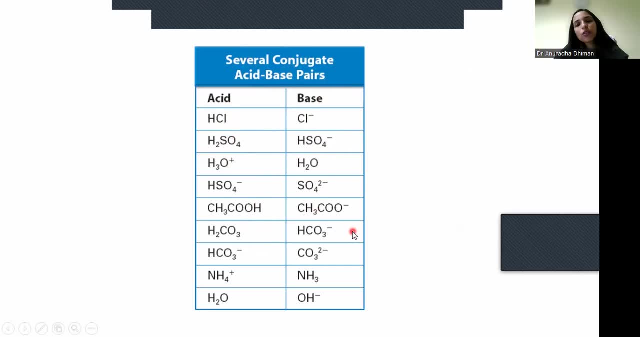 HSO4.. HSO4.. This is the same as we read: conjugate base. It is an acid and it has a conjugate base. If it is a base, then it has a conjugate acid. Okay, Learn it. Now. what is water? 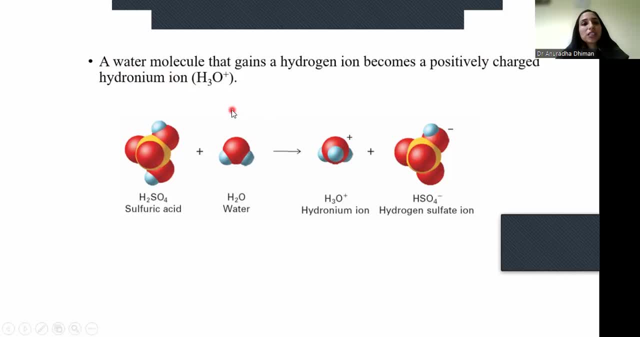 Water molecule gains and hydrogen ion become positively charged Hydronium ion. Okay, This is done. This is also the same Sulfuric acid. This is an acid and this is a conjugate base. Okay, Okay, This is the Bronsted-Lowry. 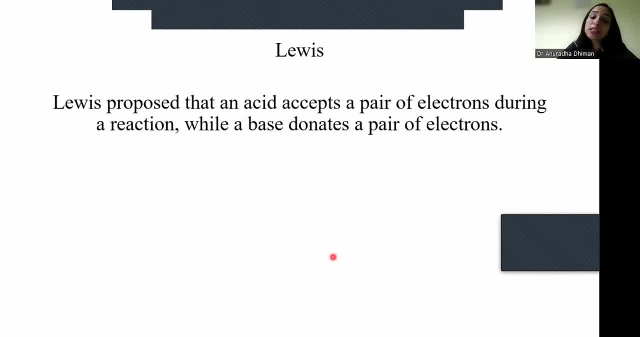 Now the next theory is Lewis theory. Now what did he propose? He says: have you seen, when we take an example, BF3.. When two atoms join with each other, there is a sharing of electron pairs. Okay, Lewis explains that. 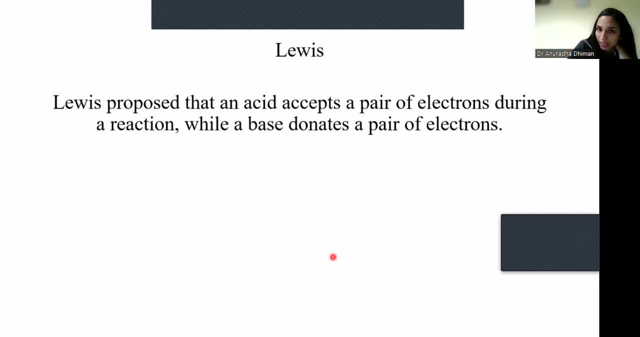 Lewis proposed a concept. According to him, what was it? The acid will accept a pair of electrons. We will accept it. The base will donate it. Earlier we were talking about protons. if you remember, Earlier I talked about OH in Arrhenius. 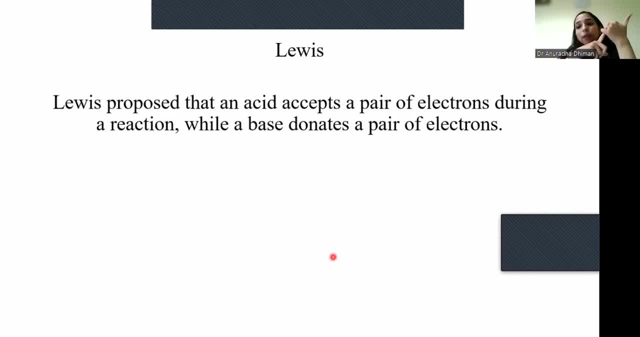 And I talked about protons in Bronsted-Lowry. Now we have come to electrons, In that the acid that will donate protons. And what is in this? They say protons and electrons. they are opposite to each other. 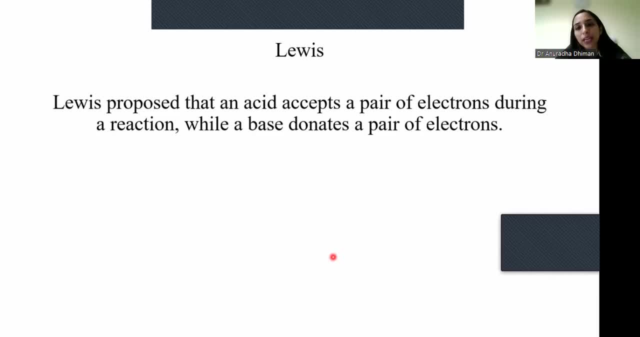 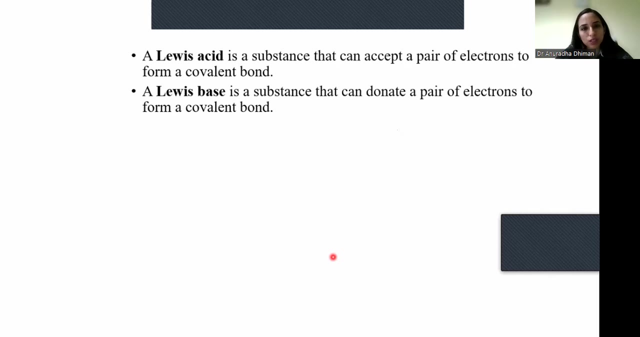 The acid accepts a pair of electrons during a reaction, while the base donates a pair of electrons. Lewis acid, A substance that can accept a pair of electrons to form a covalent bond That is known as Lewis acid. The base is its opposite. 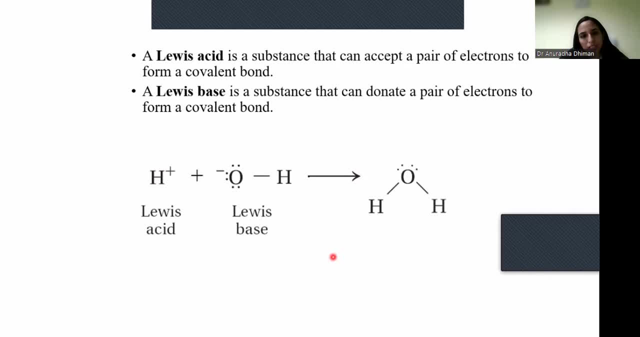 It will donate. It will form a covalent bond. Example is: this is a Lewis acid and Lewis base. Example: please write the reaction in the notebook. The rest is random. Okay, This is a Lewis acid and this is a Lewis base. 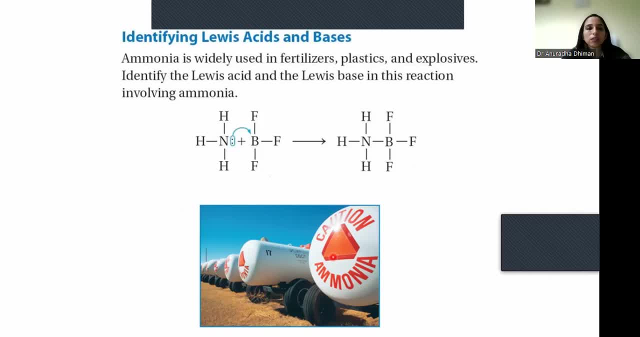 If both are joined, then H2O will be formed. Now how will we identify that this is a Lewis acid and this is a base? Okay, Ammonia is a fertiliser, plasticiser. This is ammonia and this is a. 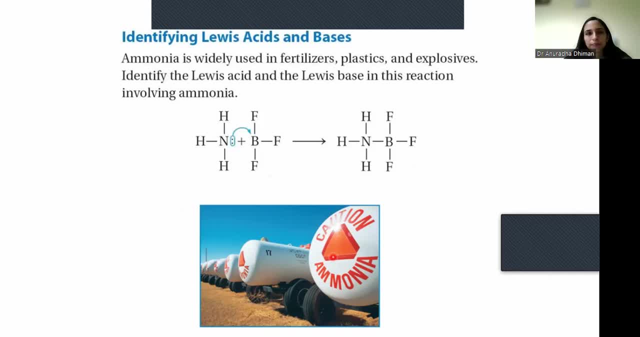 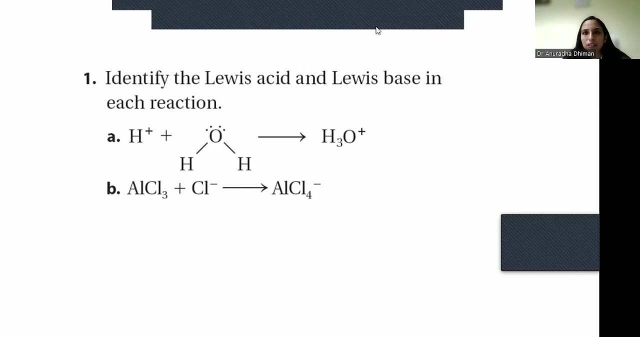 This is a Excipient BF3.. Thank you for checking out this video. If you liked it, remember to share the video with your friends who may be interested in learning more with Jesus in nature, and subscribe the channel for recent videos. 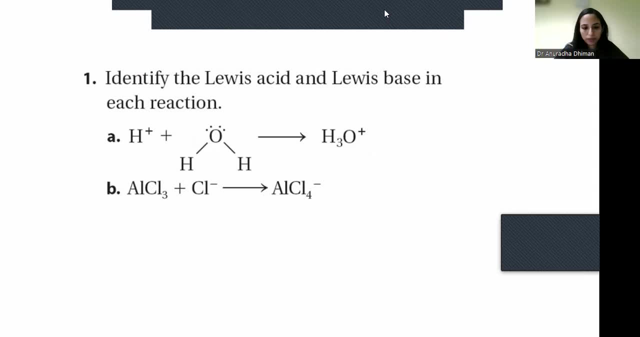 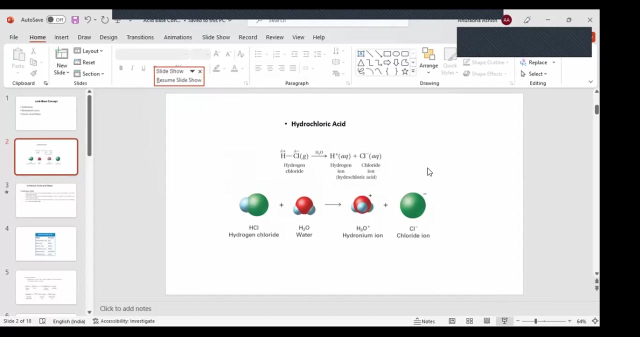 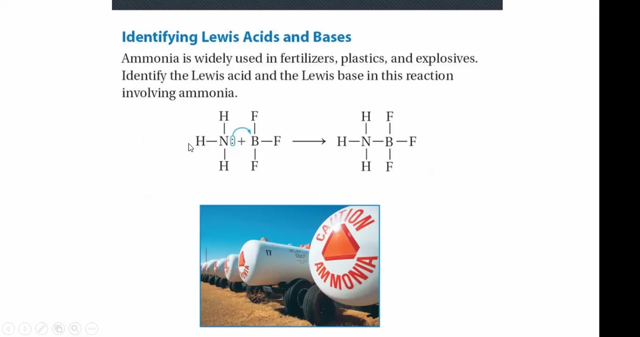 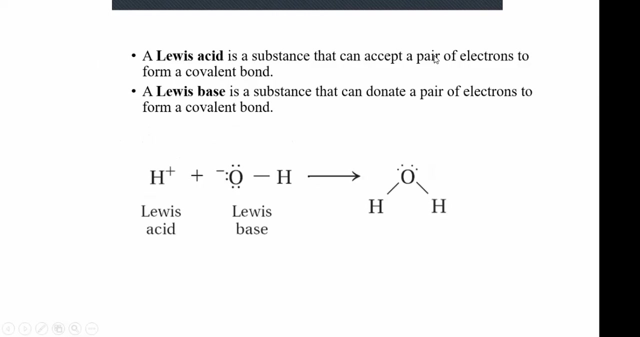 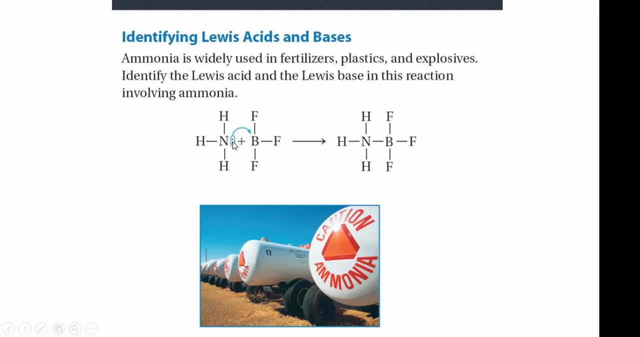 Also leave some comments. Okay, let me enlarge this. okay now, what is there in this ammonia? it reacts with boron trifluoride. now you tell me which one is acid and which one is base. I told you what is acid which accepts the pair of electrons. we will call it acid and the other is base. now you tell me which one is accepting it. this is the pair of electrons this boron trifluoride is accepting it. it means what has happened: it has become acid, it has become base, and we know that in the previous concept there was also Na3 base in it. there is also base in it. both of you see, they are also satisfying each other.